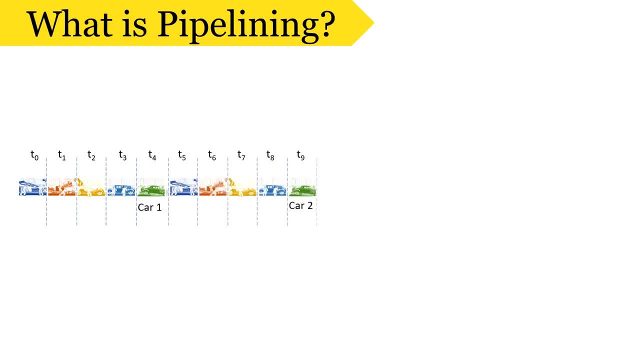 after time unit T9, they deliver the second car. Similarly, at time unit T14, they deliver the third car. and at time T19, they deliver the fourth car. Now, as we know, the process of assembling a car can be divided into 5 sub stages. Then, 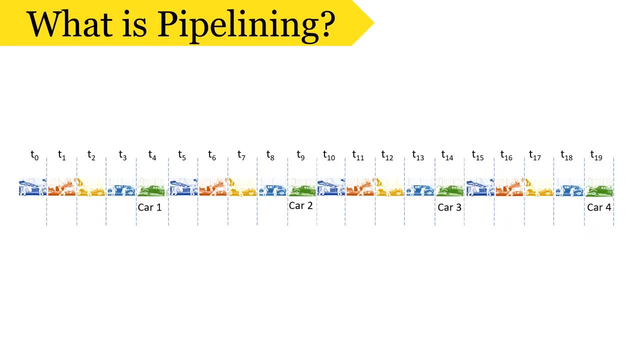 according to the concept of pipelining, we can organize the assembling of multiple cars simultaneously. In this process, we will require 5 different groups of workers, where each group will perform a dedicated task. Like group 1 will only be preparing the car chassis group. 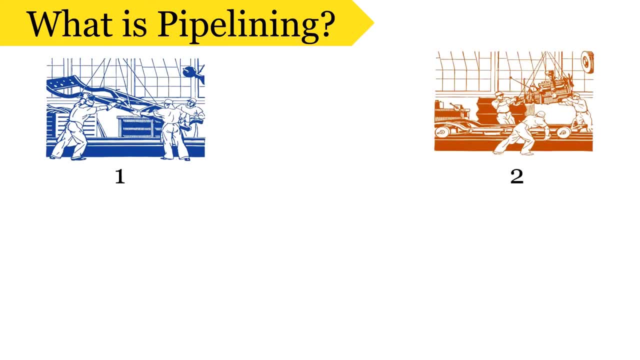 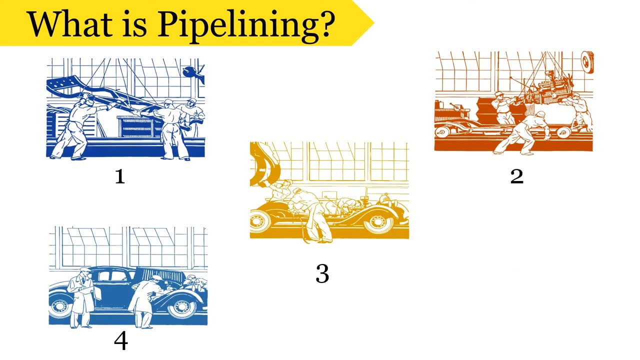 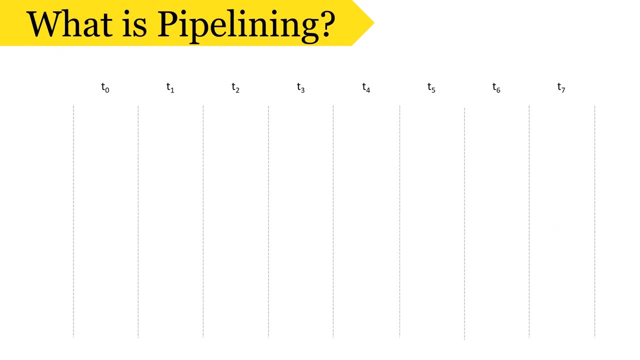 2 will only be attaching engine to this chassis, group 3 will only be adding body to this chassis, will only be painting the car body and group 5 will only perform the final check before delivering the car. Now, according to pipelining principle, at time T0, group 1 will prepare. 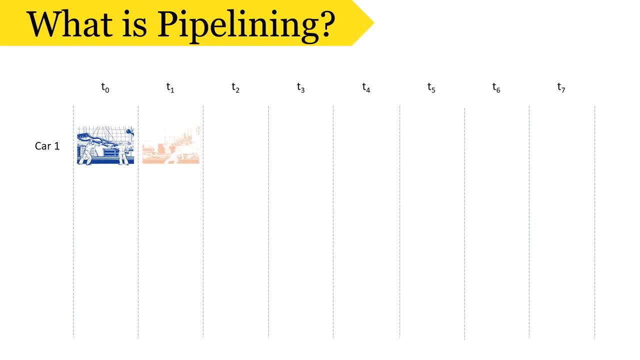 chases of car. 1. At time, T1 group 2 will add engine to chases of car 1 and group 1 will prepare chases of car. 2. At time, T2 group 3 will add body to car 1, group 2 will add. 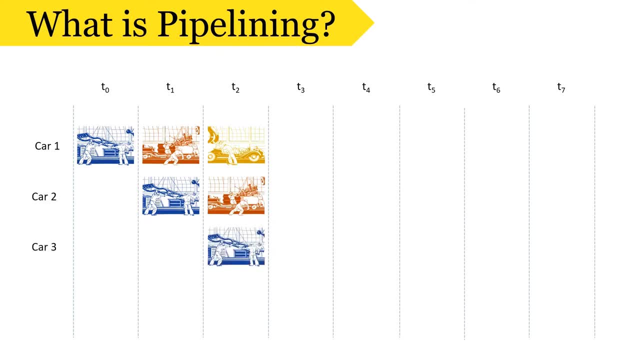 engine to car 2 and group 1 will be preparing chases of car 3.. At time T3 group 4 will paint the body of car 1, group 3 will add body to chases of car 2, group 2 will add engine to. 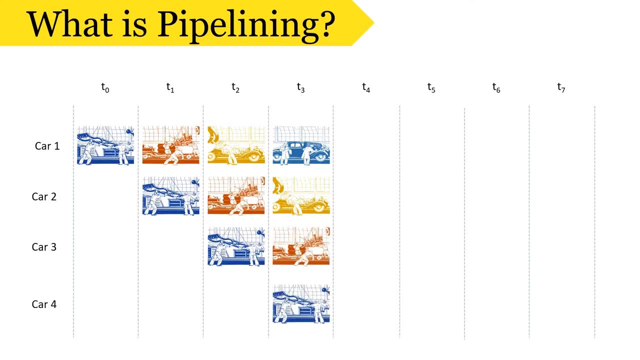 chases of car 3 and group 1 will prepare chases of car 4.. At time T4 group 5 will perform final checkup of car 1,. group 4 will paint body of car 2, group 3 will add body to car. 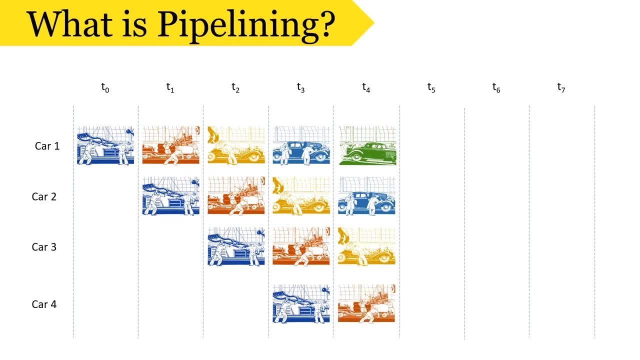 3 and group 2 will be preparing chases of car 3.. At time T4 group 5 will perform final checkup of car 1 and group 2 will add engine to chases of car 4.. So here, after time, T4- 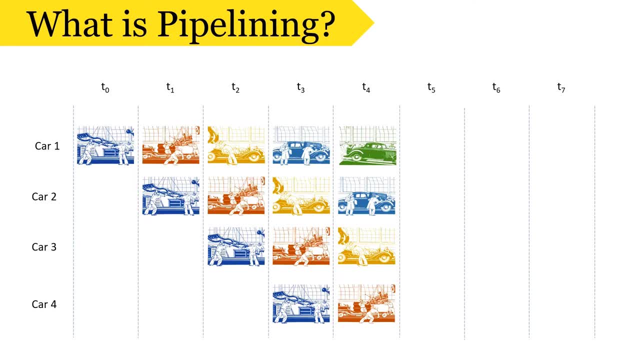 first car is delivered and after that at each clock cycle a new car is delivered. So with pipelining we can produce 4 cars by time- T7. That means pipelining increases the throughput of car manufacturing plant and if you can observe carefully then you can see the output. 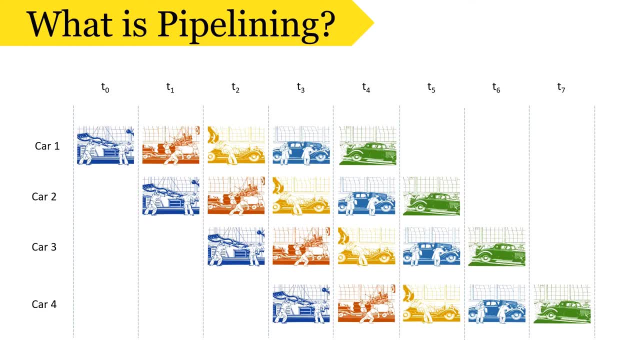 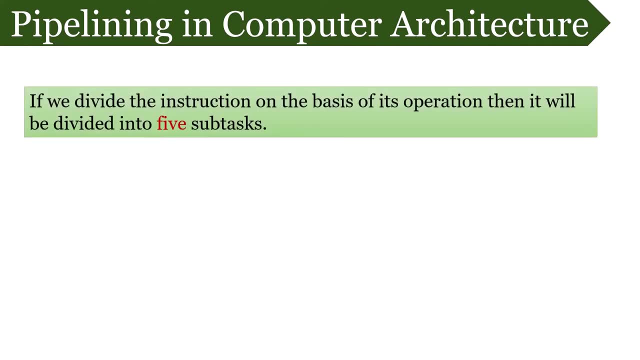 of previous group becomes input of next group. Now let us apply the concept of pipelining in computer. Here an instruction can be divided into 5 sub tasks on the basis of operation they perform, that is, instruction, fetch instruction, decode, operand fetch instruction, execution and last, 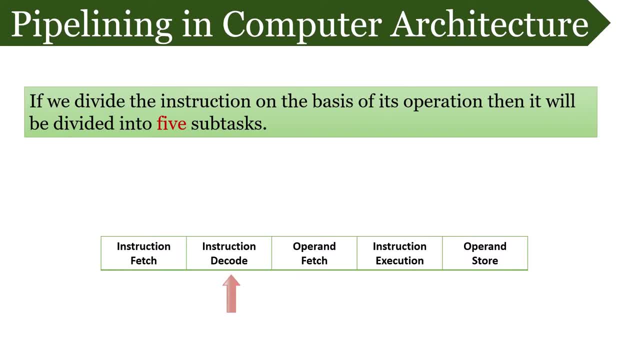 operand store. So initially the instruction is fetched, it is then decoded, after that operands of instruction are fetched, then the logical and arithmetic operations are performed on operands and lastly the result is stored on memory. After understanding the division of instruction, Let us see how n number of instruction of a process are pipelined. Lets say we have 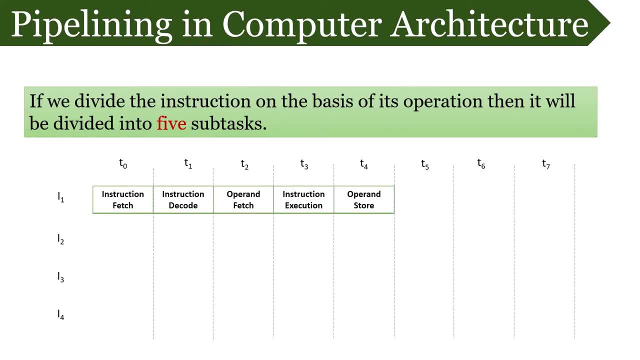 4 instructions, and first instruction is completed in 5 clock cycles. As instruction is divided into 5 sub tasks, it will require 5 clock cycles to complete execution After 5th clock cycle. in every next cycle, execution of a new instruction is completed. With this way, the hardware of 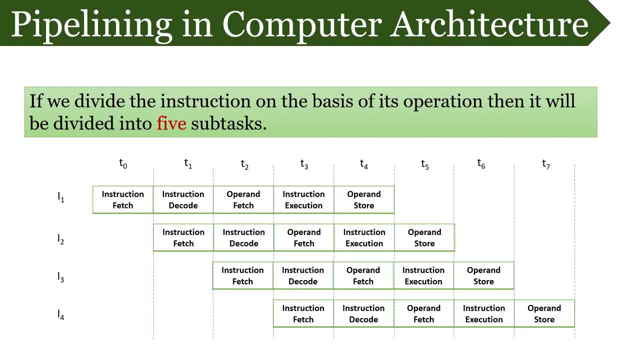 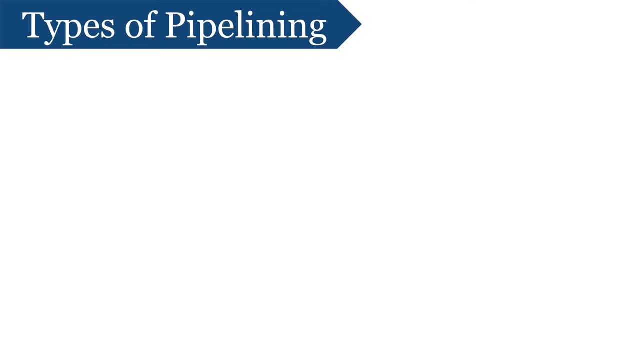 your system will never sit idle and will always keep on performing some or the other operation. Remember, the same stage of 2 different instructions will never be executed in same clock cycle. The pipelined processors can be classified depending on their functionality. First is 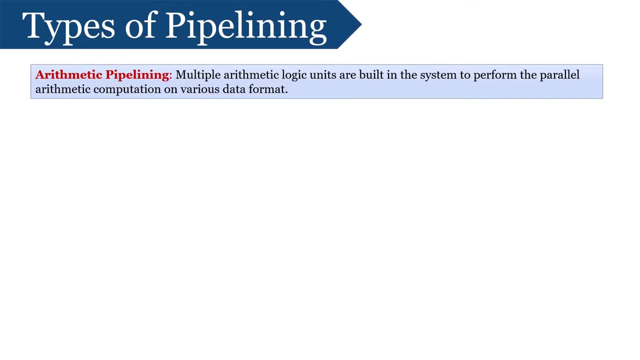 arithmetic pipelining. It is designed to perform high speed floating point operations. Here multiple arithmetic logical units are built in system to perform parallel arithmetic computations on various data format. Next is instruction pipelining. Here the number of instructions are pipelined and execution of current instruction is overlapped by the execution of subsequent. 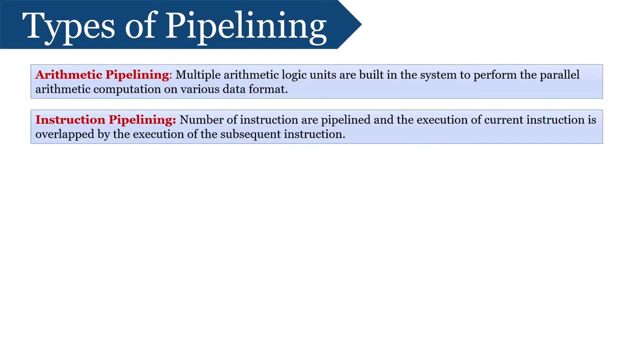 instruction. It is also called as instruction lookahead. Next is processor pipelining. Here the processors are pipelined to process same data stream. Thus, data stream processed by the first processor is reprocessed by the second processor and the result of second processor is reprocessed by the third processor. Next is unifunction versus multifunction pipelining. 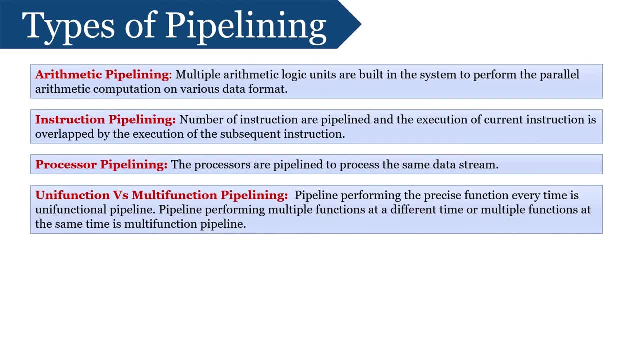 The pipelined performing precise function every time is unifunctional, Whereas the pipelined performing multiple functions at different time or multiple functions at same time is multifunctional. Next is static versus dynamic pipelining. The static pipelining 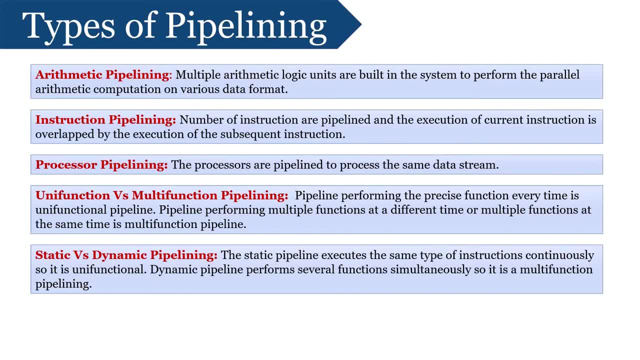 perform a fixed function each time. Thus it is also known as unifunctional. The static pipelined execute the same type of instructions continuously, and frequent change in type of instruction may vary its performance. However, dynamic pipelined perform same type of instructions. 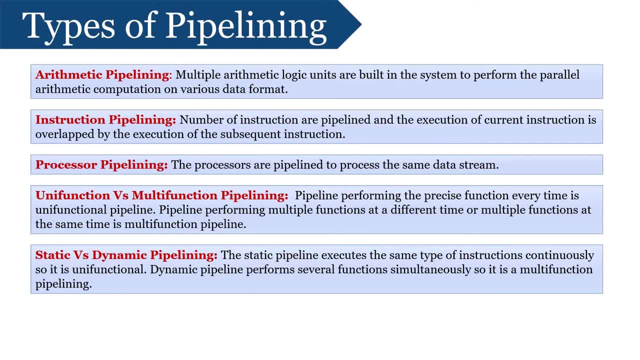 Several functions simultaneously. Thus it is also known as multifunctional pipelining. Next is scalar versus vector pipelining. Scalar pipelining processes the instruction with scalar operands, whereas vector pipelined processes the instruction with vector operands. Now, sometime a pipelined has to stall or stop due to some reasons. This is called pipelining. 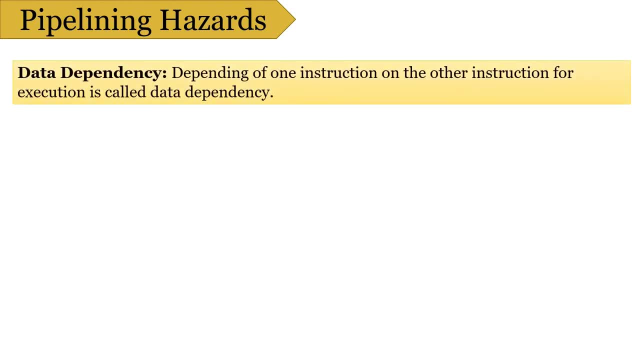 hazard. The first hazard is data dependency. Depending of one instruction on another for execution is called data dependency. In the example below you can see that result of add instruction is stored in register R2 at clock cycle T4.. But R2 is also an operand of next subtract instruction, whose operand 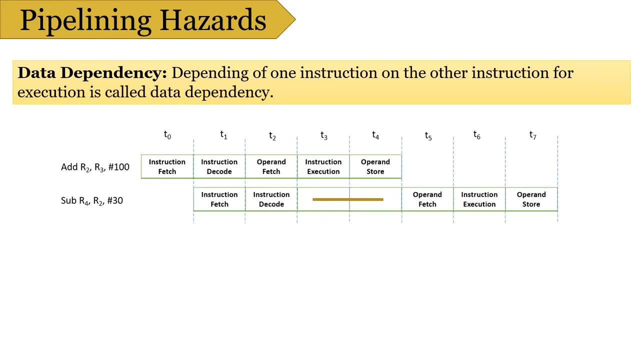 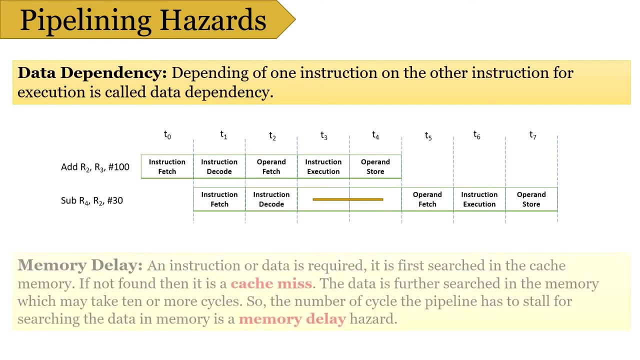 fetch takes place in clock cycle T3. But as the correct value of R2 is available at T4, so subtract instruction needs to stall for two clock cycle. Thus, depending of one instruction on another for data is called data dependency. The next is memory delay. When an instruction or data is required, it is first searched in. 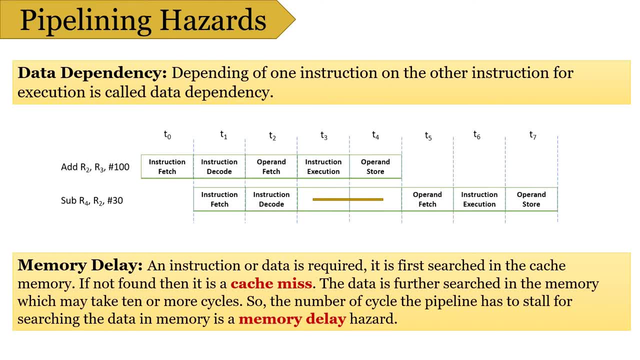 the cache memory and if it is not found there it is a cache miss. The data is further searched in the memory, which may take ten or more clock cycles. So for that number of cycle pipeline has to stall and this is called memory delay hazard. The cache miss also result in delay. 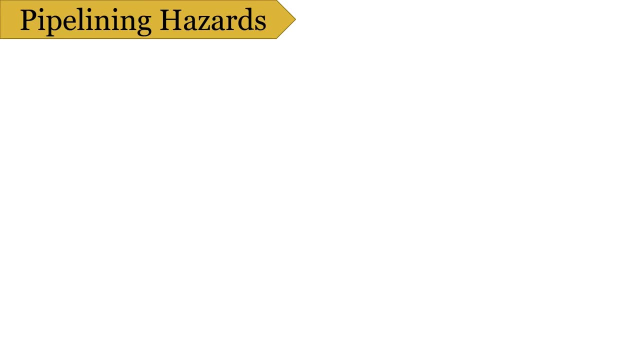 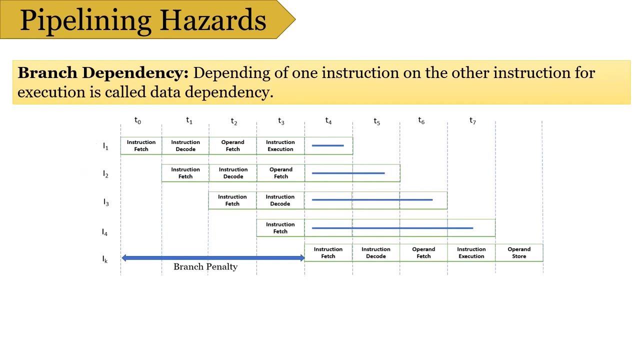 of all the subsequent instructions. The next hazard is branch delay. Suppose there are four instructions pipelined- i1, i2, i3 and i4 in a sequence. Now the instruction i1 is a branch instruction and its target instruction is ik. The processing starts and 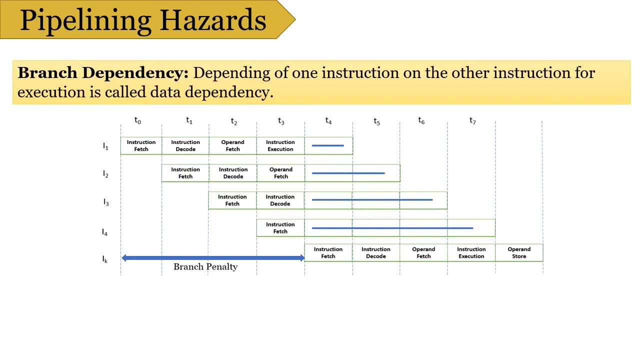 instruction i1 is fetched, decoded and target address is computed at forth stage in cycle T3.. But till then, instruction i2, i3 and i4 are fetched in cycles 1,2 and 3, before the target branch address is computed.